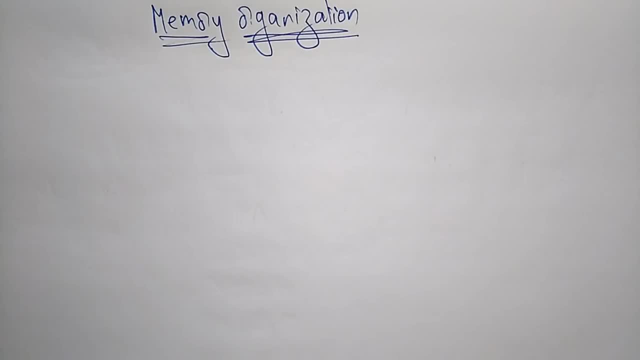 Hi students. coming to the next topic, that is, memory organization. So how the memory is organized in the computer, Let us see the internal. There are different types of memories that will be present in the system, in the computer, So that maybe you can add the external memory devices, or internally you are having different memory devices. So let us see what are the different types of memories that are present in a system. So here we had seen the memory. 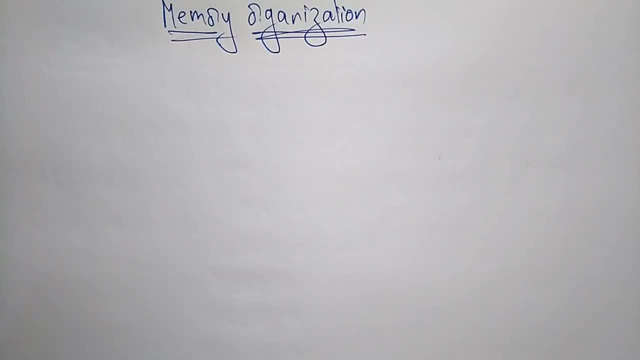 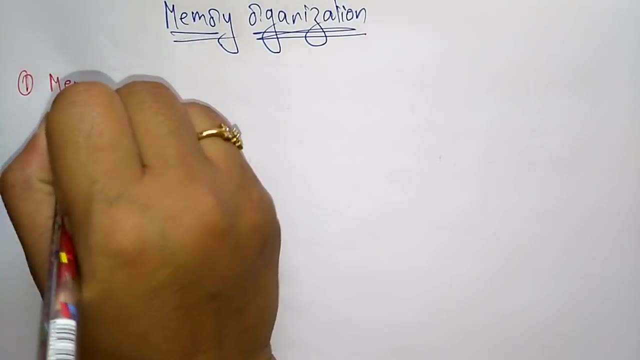 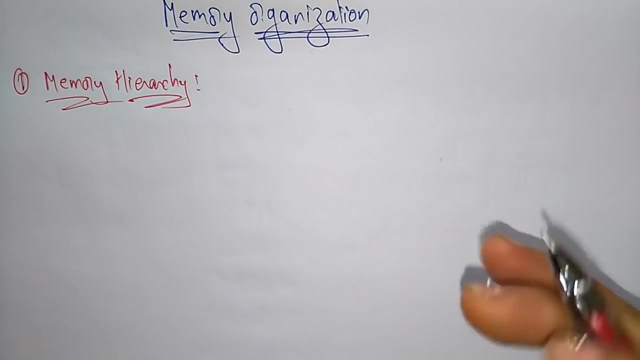 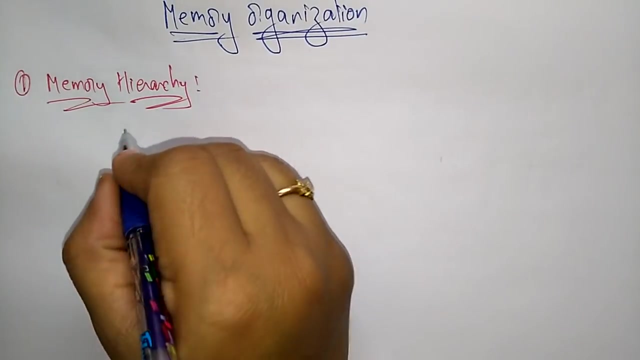 hierarchy and the main memory and we will see different high speed memories in this memory organization. So first let us see what is the memory hierarchy, What are the different memories that are present in the system and what is the hierarchy of that memories. A computer memory should be fast, large and inexpensive. A computer memory- whatever the memory that is used in the computer. 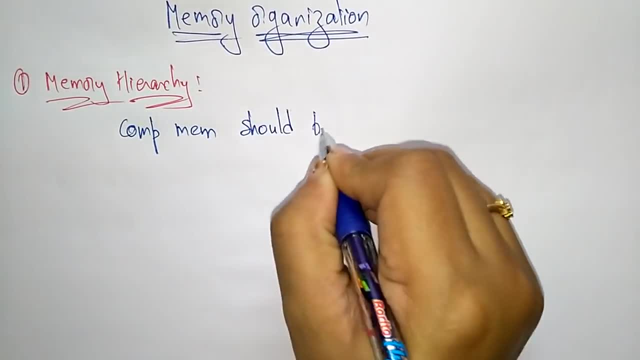 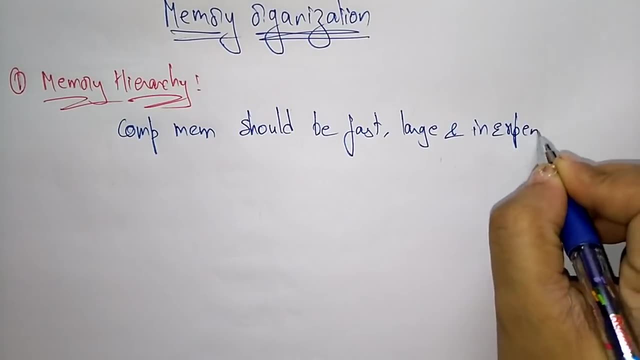 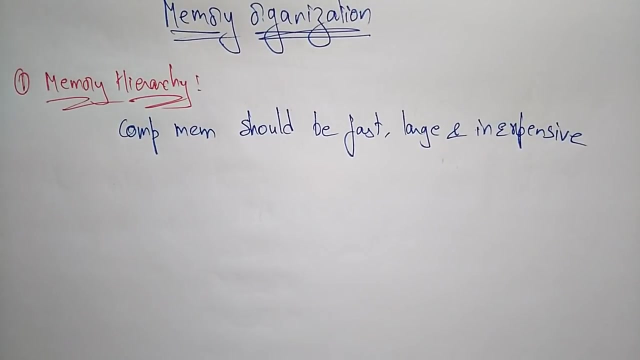 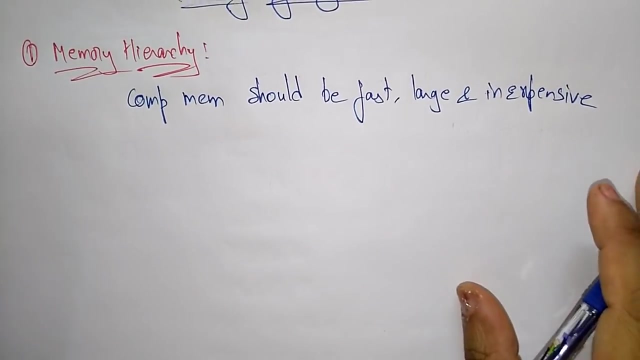 Should be fast, large and inexpensive. Okay, so the fast memories can be achieved by SRAMs, whereas large memories can be used by DRAMs. So RAM is nothing but a random access memory. So let me explain the hierarchy is obtained. How the hierarchy is obtained. The memory hierarchy is obtained by: 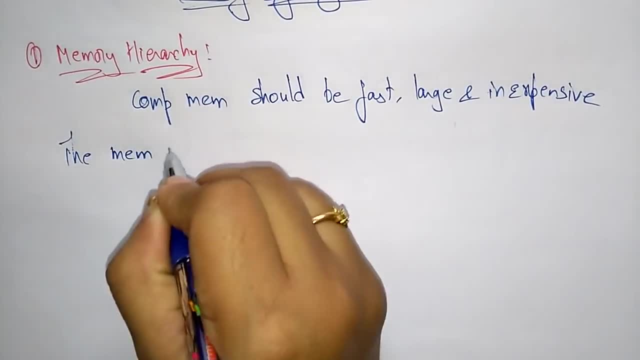 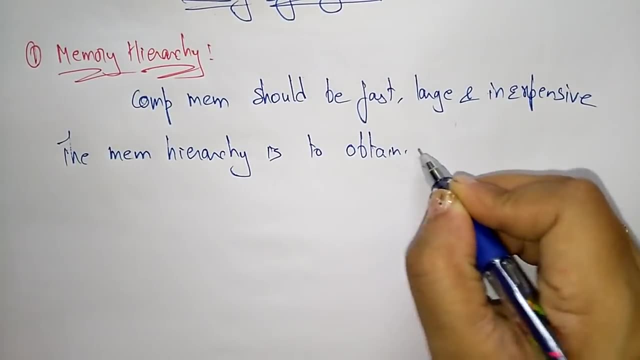 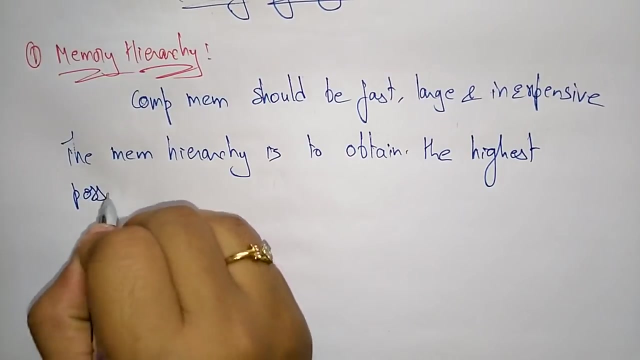 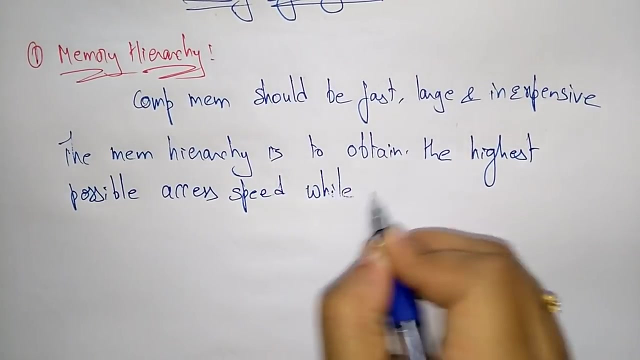 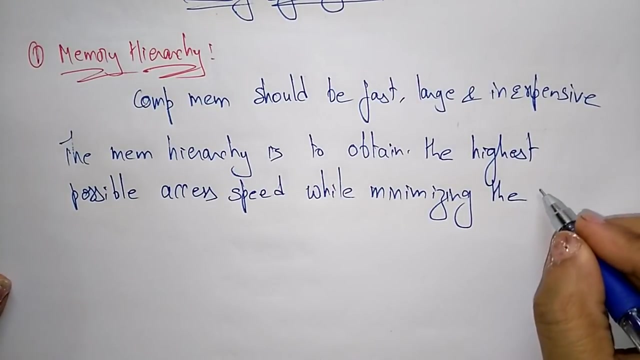 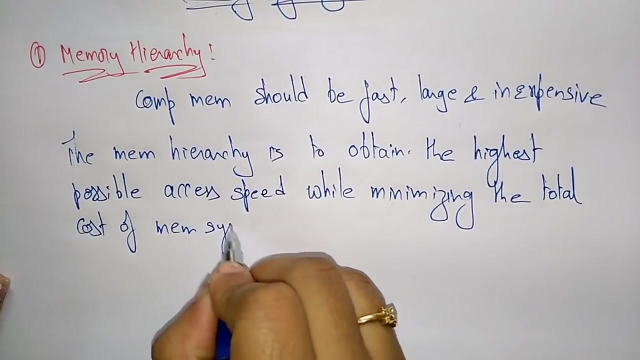 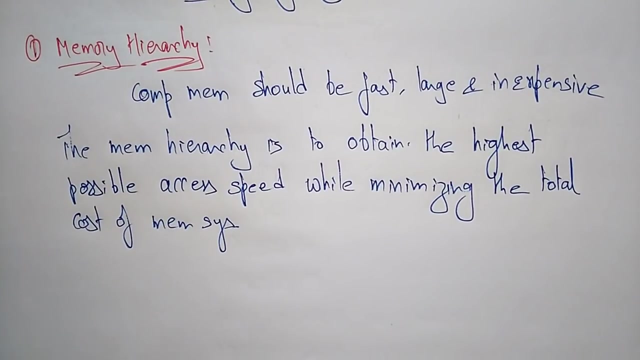 The memory hierarchy. The memory hierarchy is to obtain the highest possible access speed, the highest possible access speed While minimizing the total cost of memory system system. total cost of memory system. so the memory hierarchy is obtained, the highest possible access speeds while minimizing all the total cost of memory system. so how the memory hierarchy will. 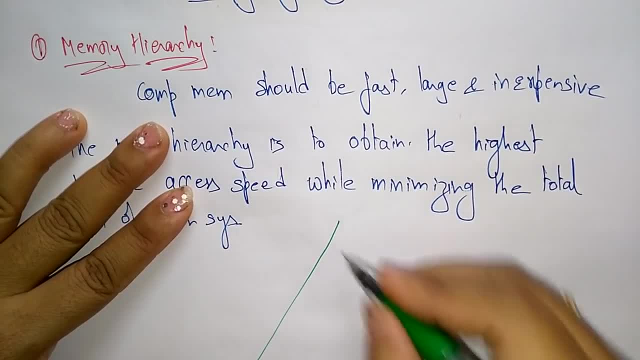 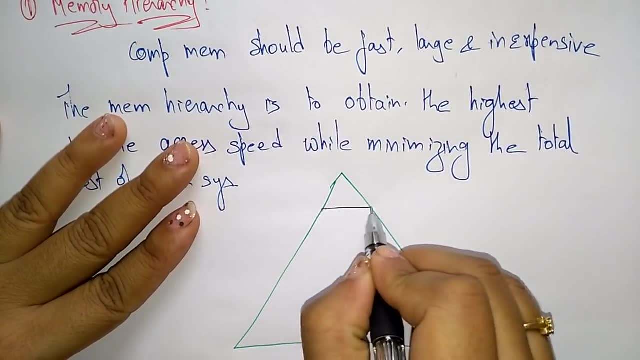 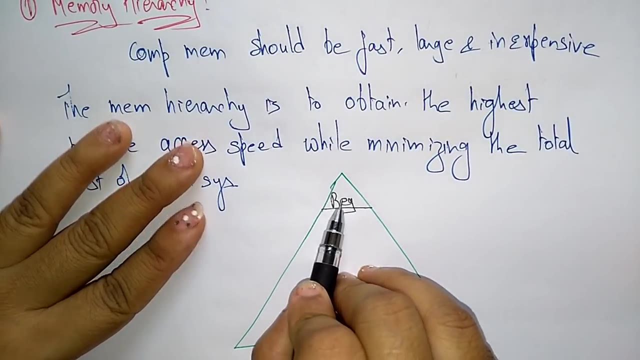 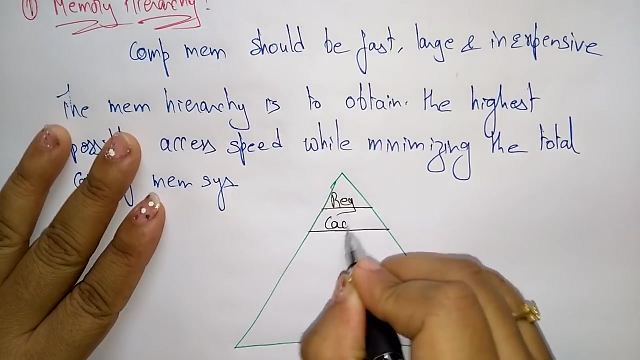 be represented. so let me take a simple diagram. so the different memories that are present in the system. computer system is: first is the register. use it to store a small amount of data, but it is the topmost memory device, which is a fast, very fast device cache. 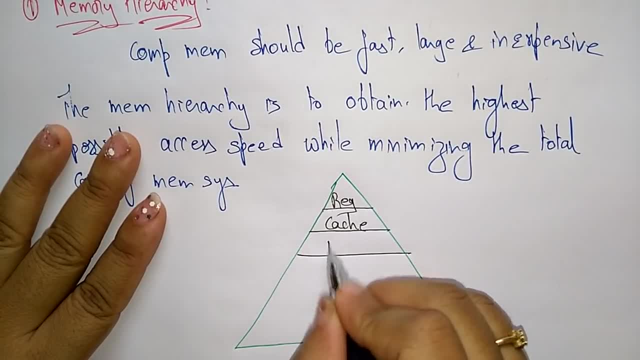 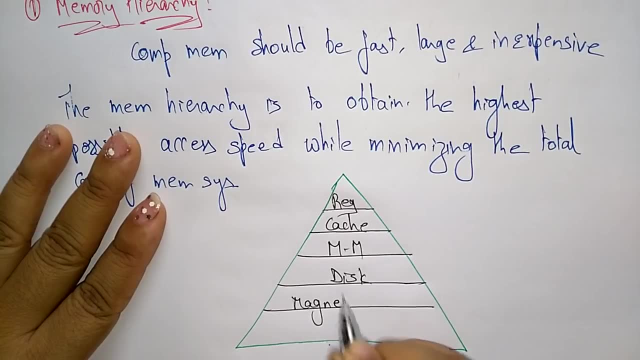 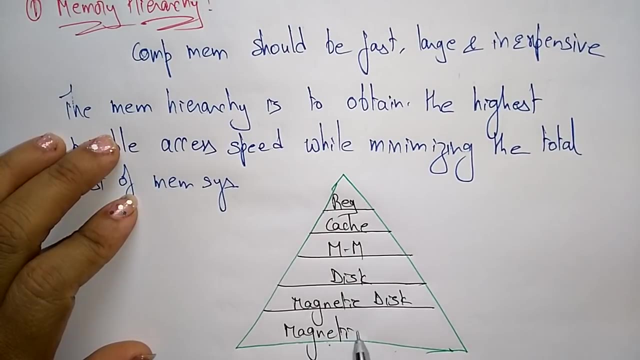 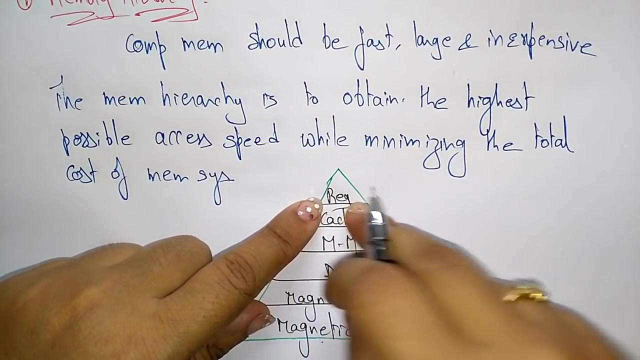 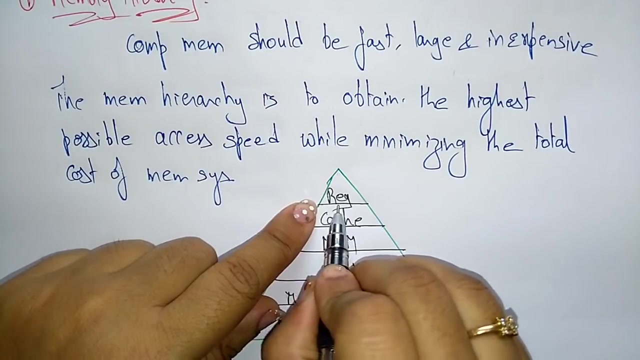 next, main memory disk, magnetic disk and magnetic tapes. so the hierarchy will be like this. so this is a register which is very close to the processor. so whatever the data that has to be executed by the processor at that time, that data will be stored in registered. a register is a very small device. it only stores a small amount. 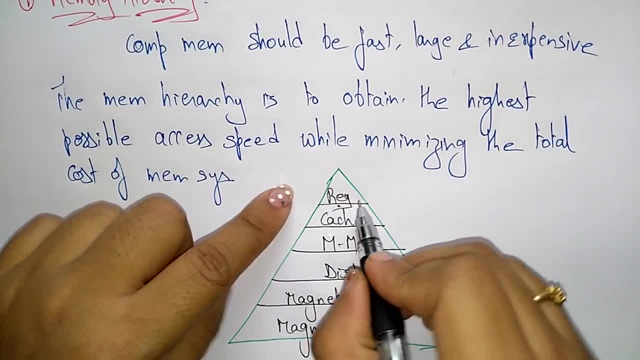 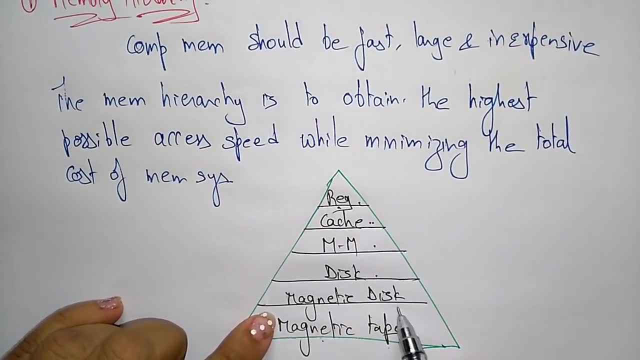 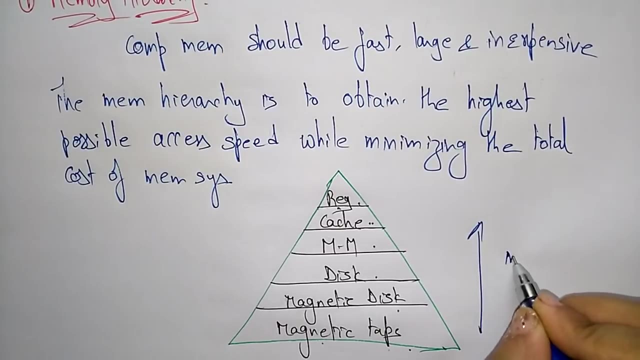 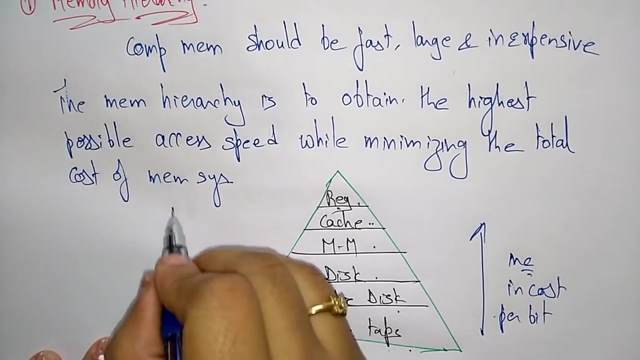 of data but very faster accessing: register cache. next fast accessing is a cache. next fast will be the main memory. next is a disk, magnetic disk and magnetic tape. so here the increase in uh in cost per bit. here the cost per bit will be increased. so whereas here, when you coming from top to bottom, it increase in capacity and access time. so here 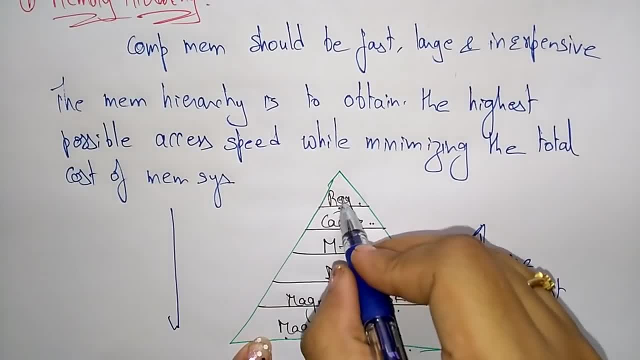 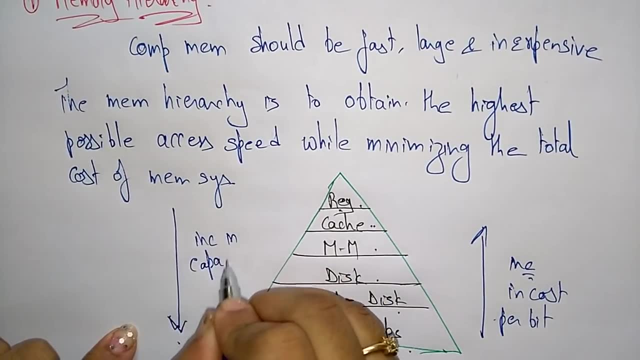 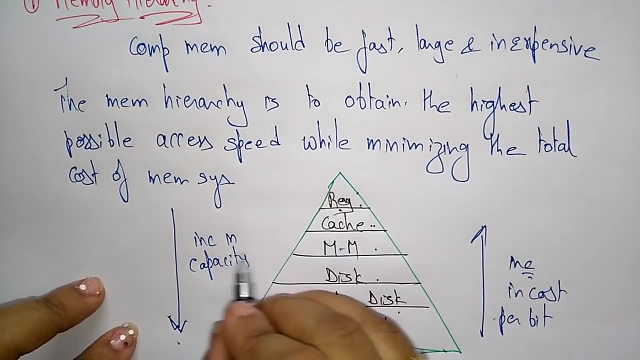 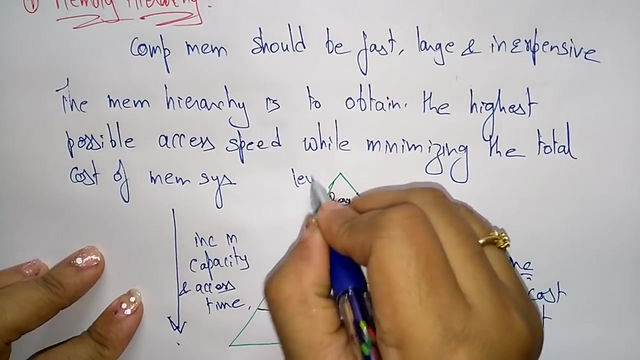 the magnetic tape access time is more when compared to the register. so that's why here the arrow mark is down here: increasing capacity. so when compared to the register, magnetic tape tape capacity is more, but the fast is the registers, increasing capacity and access time. okay, so this you call it as a level 0 and this is a level 5. 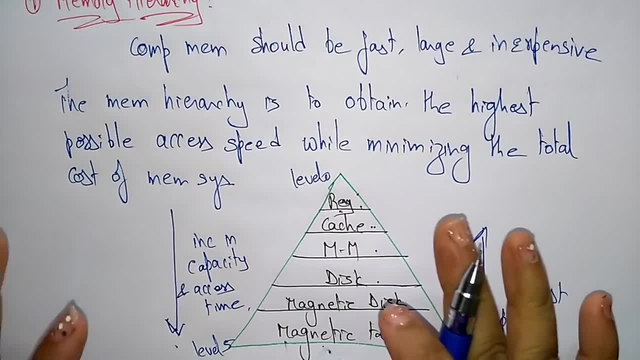 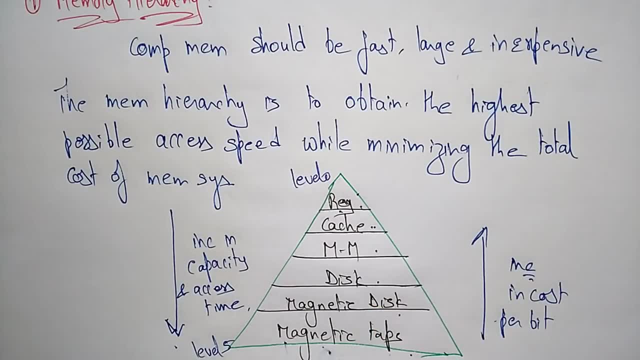 so this is the different hierarchies of the uh memory. so these everything will use by the computer, so a computer will be the same. so this is the. it is called linear memory. ok, so the system should be a fast, large and an inexpensive can be decided based on these memories chosen by. 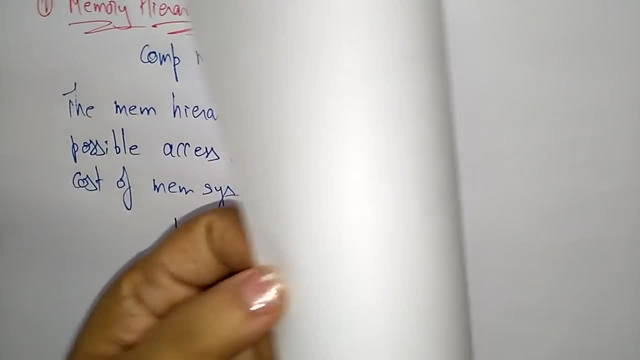 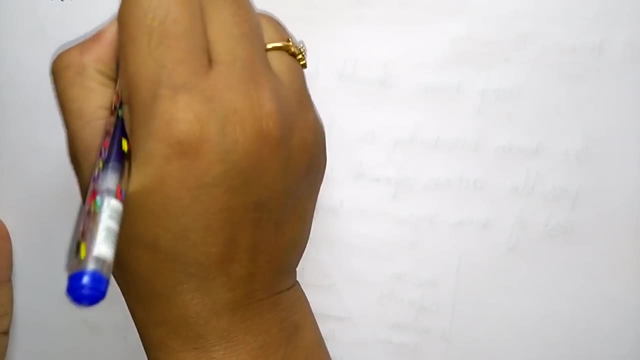 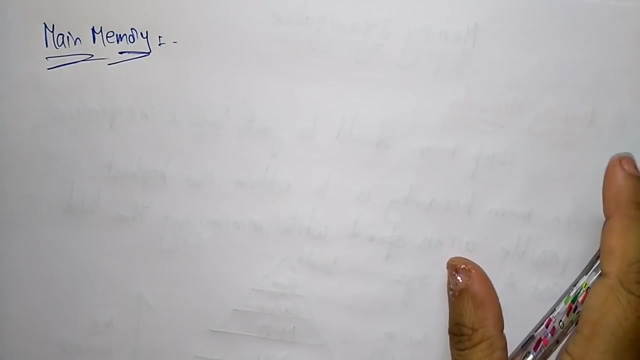 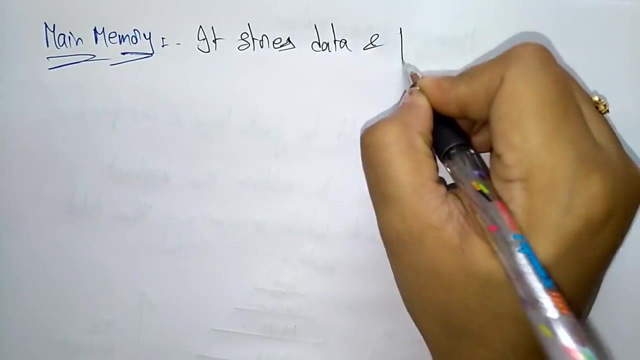 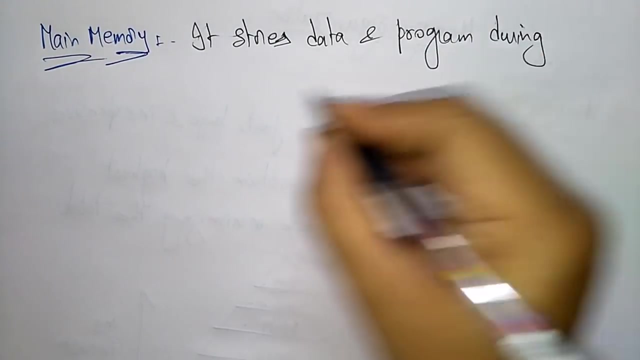 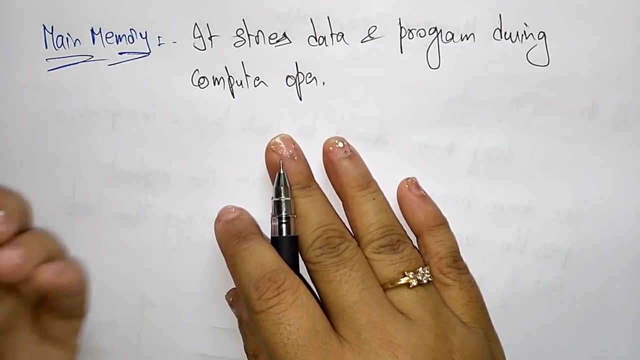 the user. okay, now let us see what is a main memory: main, main memory, so the main memory. it stores data and program during the computer operations. so main, it stores data and program stores the data and program during computer operations. so whenever the computer is doing the operations, the main memory is used to store the 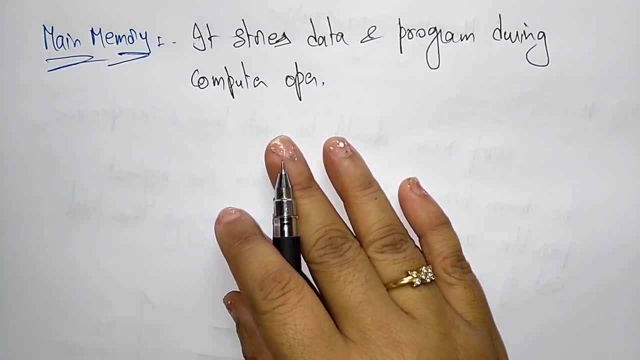 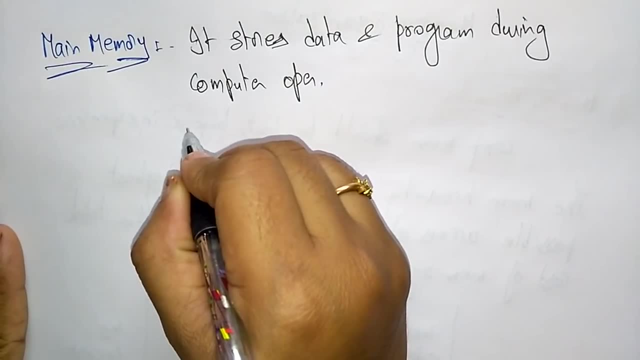 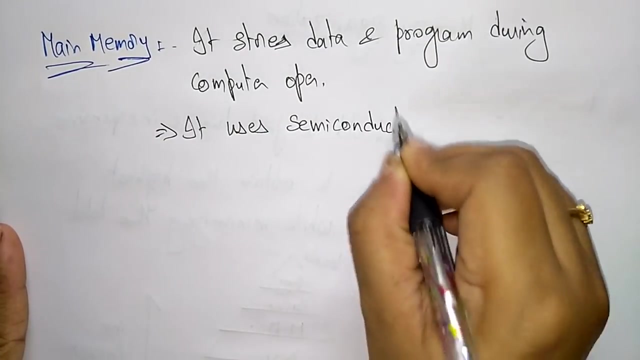 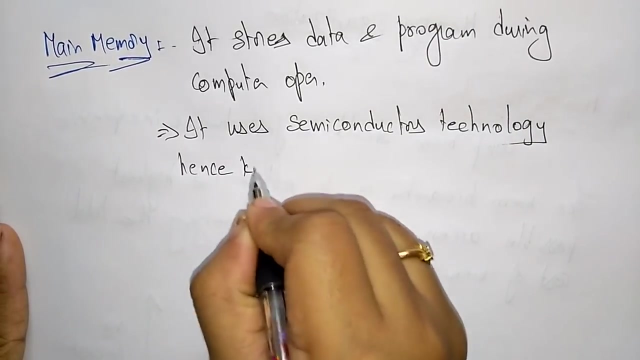 data and the programs. so the main memory may be divided into two types: volatiles and non-volatiles. let me explain the monos election. so the monos election, a selected date and method. so system me explain that. So it uses this main memory, uses semiconductors technology, Hence known. as semiconductor memory. So it uses a semiconductor technology. That's why we call this main memory as a semiconductor memory. So the semiconductor memory is divided into two types That memory, whatever we are taken, that may be a volatile memory and non-volatile memory. Non-volatile. 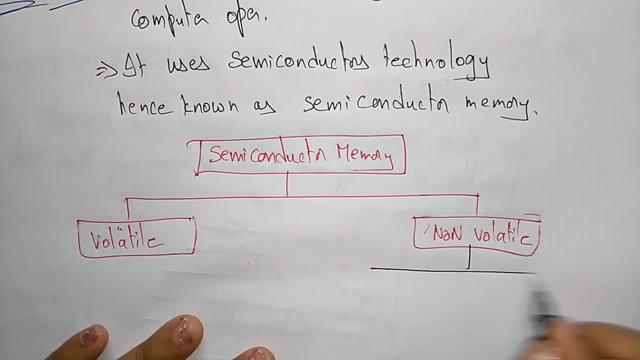 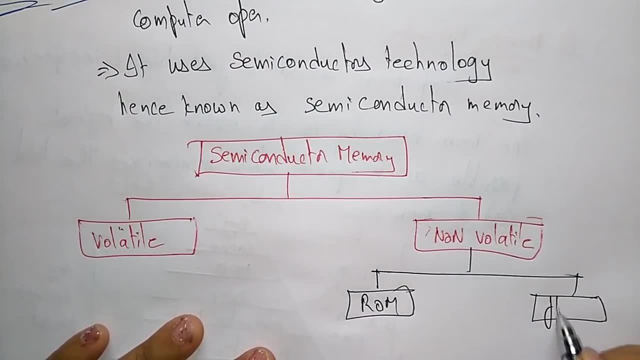 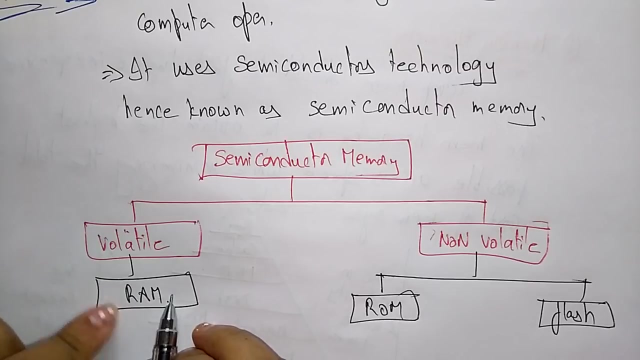 memory. So the non-volatile may be is a two types, ROM and flash, Whereas volatile memory is RAM, random access memory. Volatile means whatever the data that is present will be erased whenever the system is off power. 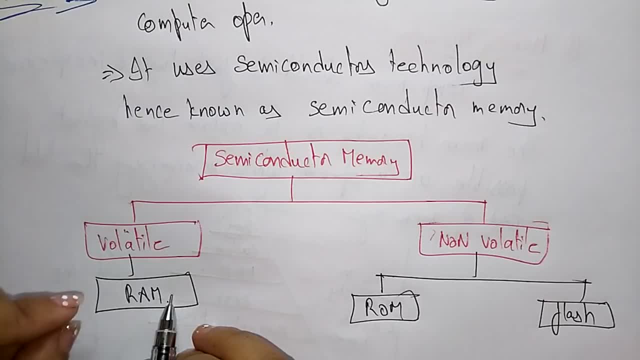 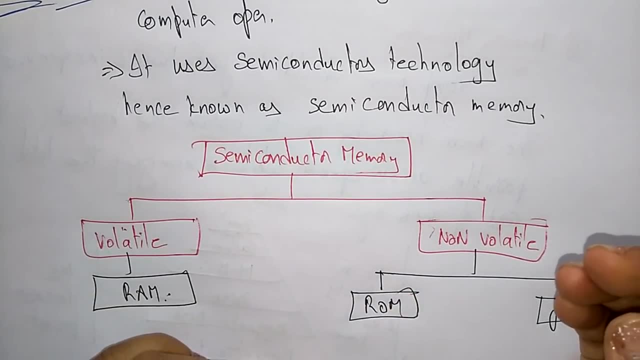 supply is off or if you close the program, that data that is present in the RAM will be erased. Volatile means the data will be erased. Non-volatile means it is a permanent data. It won't be erased. Okay, So it is a permanent. 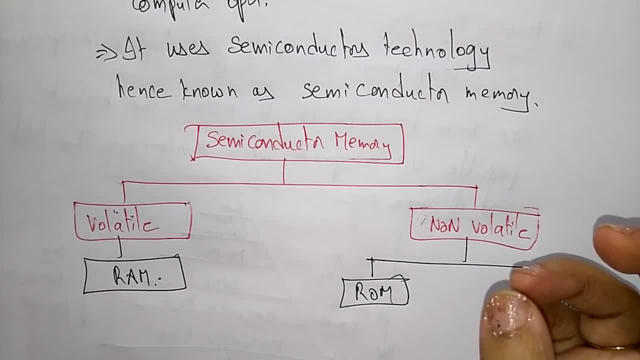 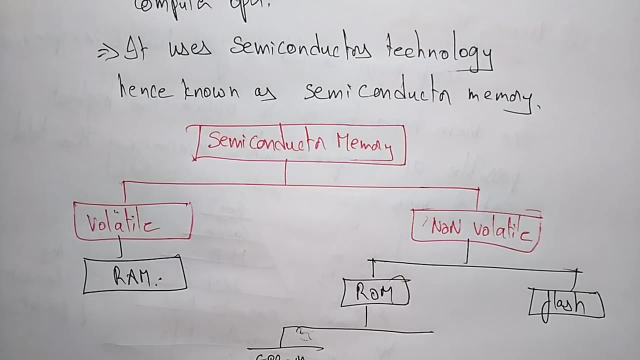 data Non-volatile stores. a permanent data Volatile stores the data that is temporarily So that data is erased will be removed whenever your system is off or if you close the files. So again, this ROM may be different types: EPROM, PROM, programmable read-only memory. 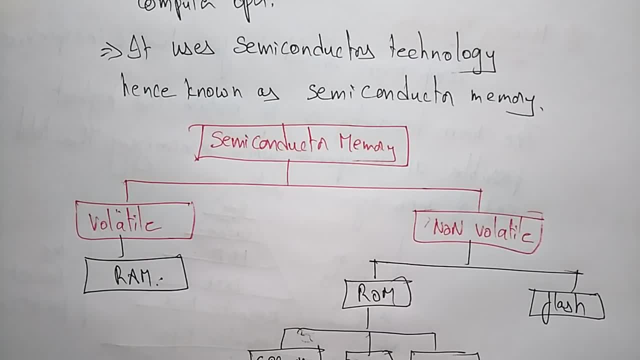 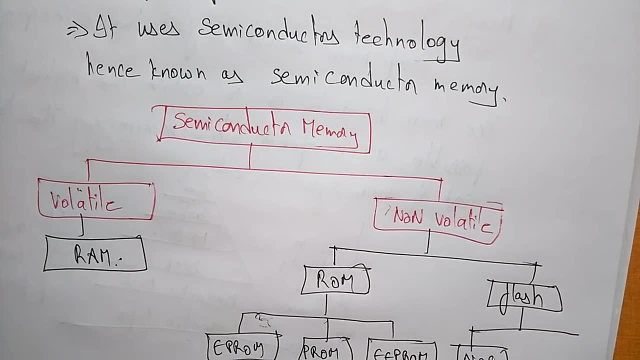 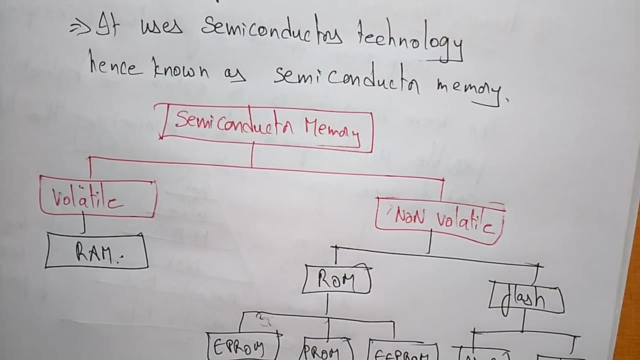 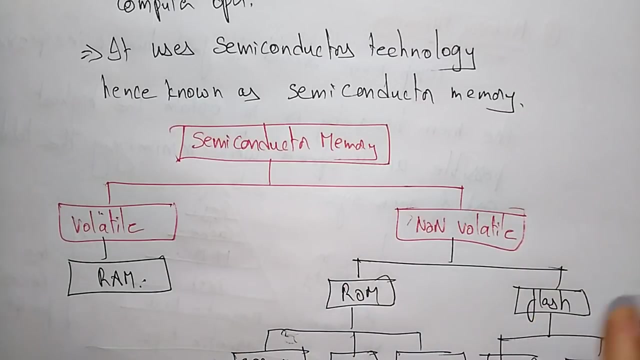 electro ko节, well programmable, read-only memey double EPROM. So this of the different types of ROM upcoming to the flash, NOR and NAT, so NAND, NAT, So these are the different types of main memory, So the main memory that is any음, a country of memories may. be maybe a volatile, or it may be do- dé ou non-volatile, or it may be回 cur Ching memory. I should come back later on for the next go. this is the flash value. but the FiME to the Bloos Food stole the Jelly piles name, remember. I have completed the level N and bizgot, But okay. So now I'm going to take a set-up to protect the carro's, So I'm 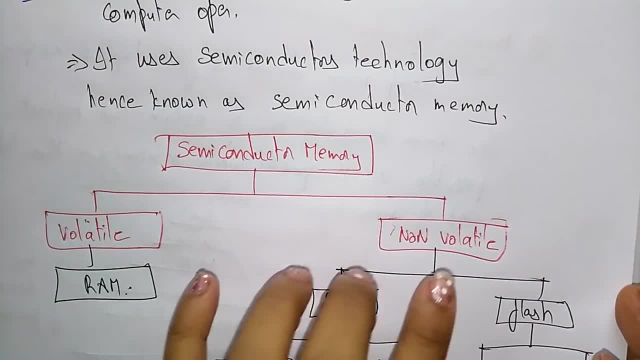 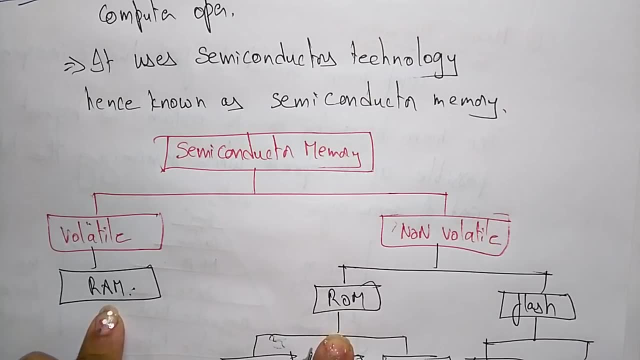 use. the non-volatile means both will be used. volatile will be used and non-volatile will be used, so both should be present in the system. so whenever you are designing the system- computer system- the ram should be there and the rom should be there. rom is used to store the permanent.